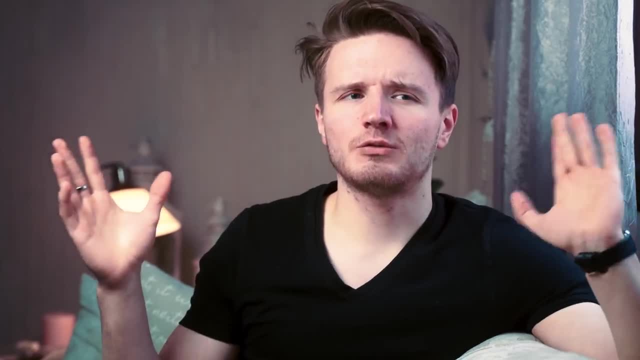 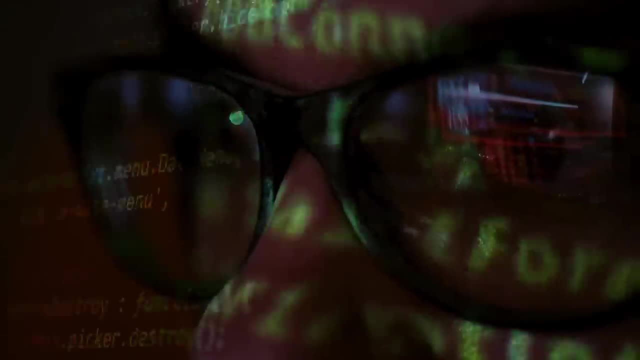 coding even was. I just had this vague idea that it's something related to typing complicated stuff on a computer to get it to do something, And that's essentially what programming is. It's you speaking to a computer to tell it what to do. But a few months ago I had absolutely 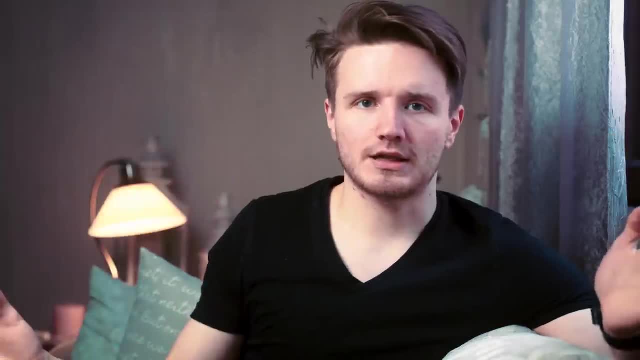 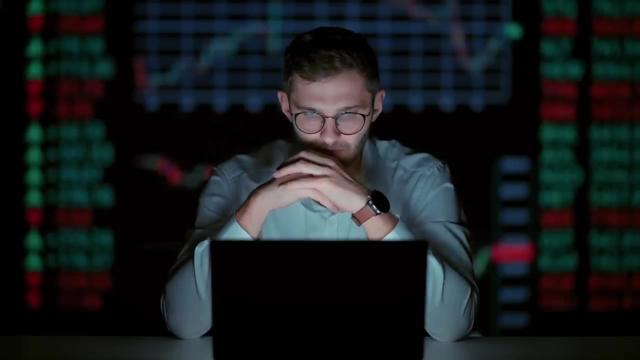 no idea what it is, what all the other languages do, anything related to it. I got the idea of learning how to code after I graduated from university with an economics degree. Now, most people who do economics end up doing investment banking, consulting and these. 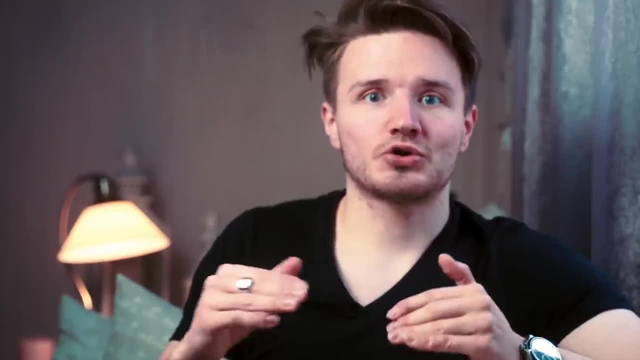 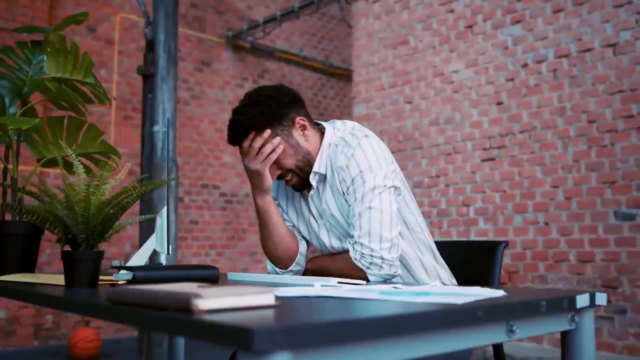 types of things, And I did an internship at a bank. But, long story short, I absolutely hated banking. I wasn't passionate about economics and I certainly wasn't passionate about working in finance or many of the other industries where economics grads usually go to. I could have easily done it and gone on to make a 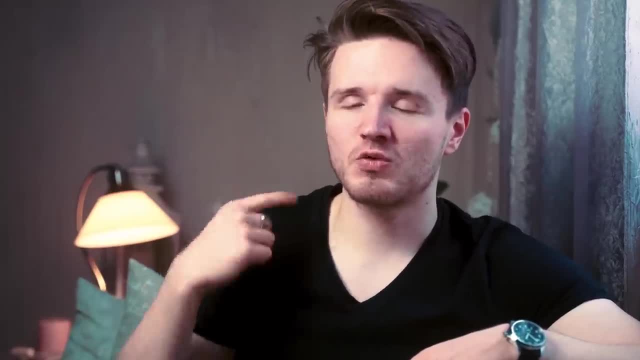 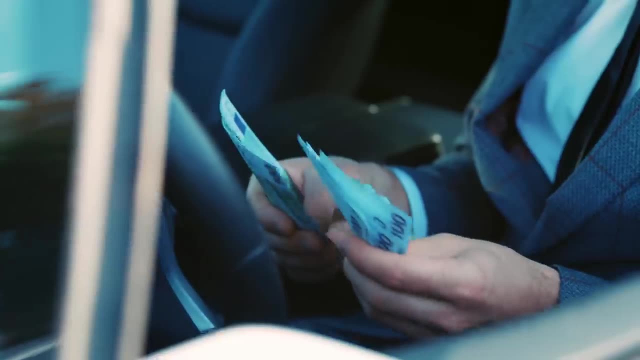 lot of money as a banker, but I just hated the lifestyle. The work wasn't inspiring to me. So it was clear that I needed a new plan. So why did I decide to learn coding? I wanted to find an industry where I could still make a lot of money but also have a more humane 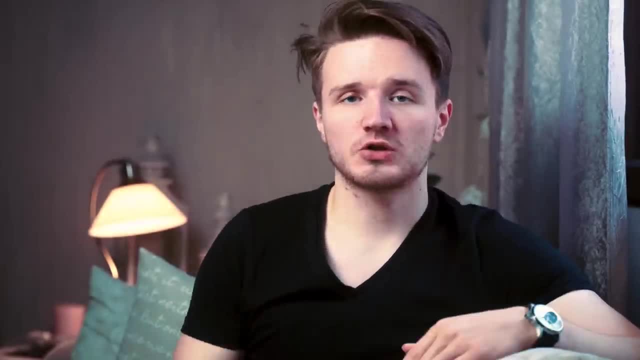 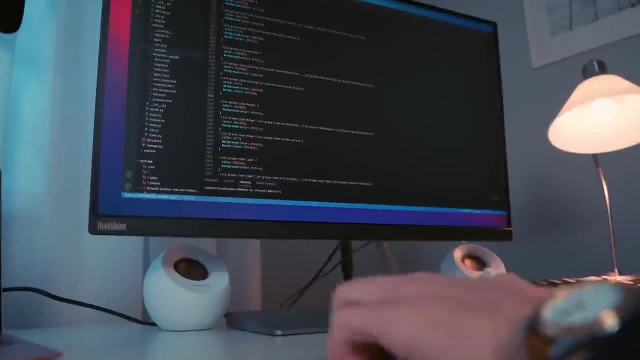 lifestyle and work on problems that I'm actually excited to work on. So I discovered software engineering. So I learned that, in order to become a software engineer, all you really needed was know how to code. So I went on Google, typed how to learn how to code, and I ended up starting. 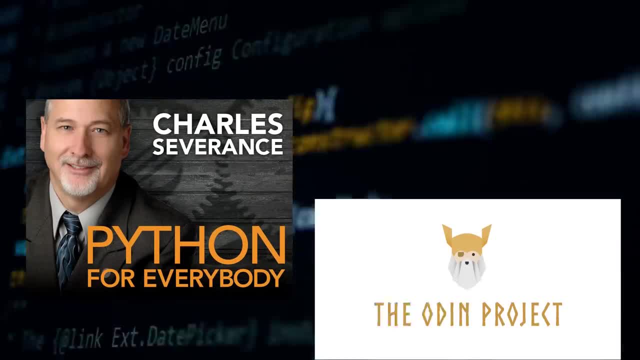 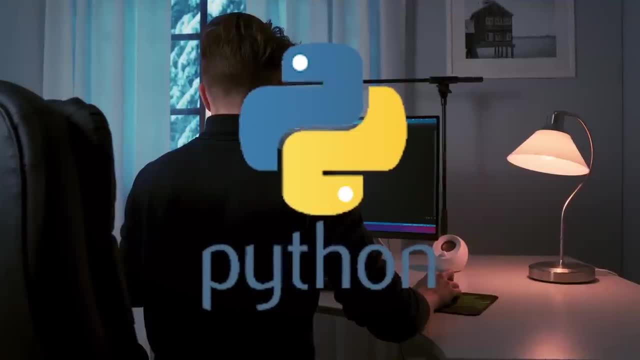 with resources called Python for Everybody and The Ori Project. These are both completely free resources that I found online. The former introduced me to Python, one of the most popular programming languages of today, and the latter introduced me to web programming, So I learned. 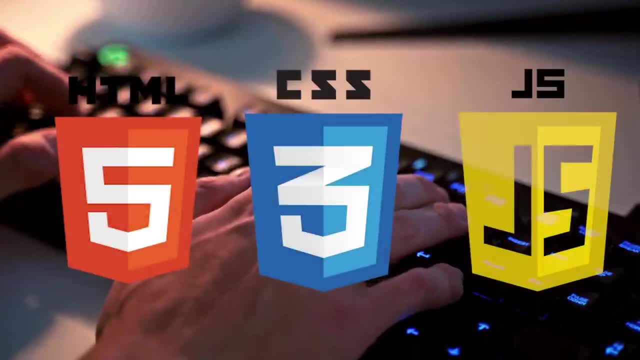 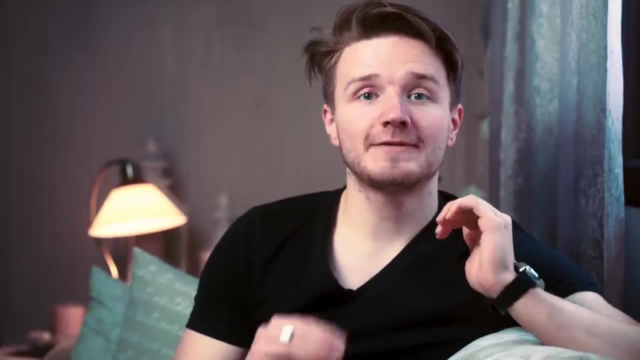 how to build a web page using HTML, CSS and JavaScript, And some of the resources that I found were really useful. I learned a lot about how the internet works and what it actually means for you to open a web page on your computer, And I was absolutely fascinated. 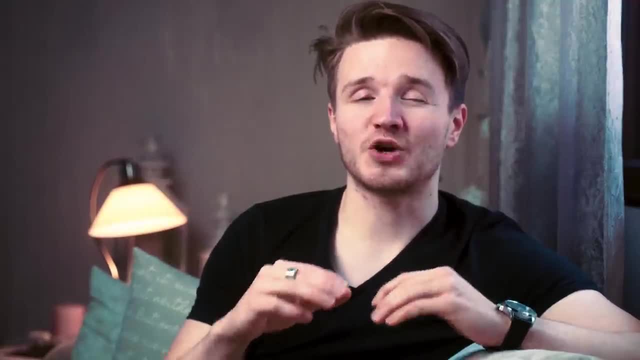 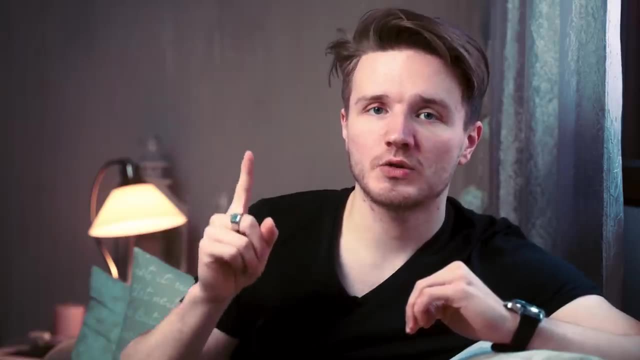 by all of this. So the next step was to take a proper introductory course in computer science, And I decided to go for Harvard University's CS50,, which you can do for free on edX, And I've done a review on it which you can watch right here. Long story short: it's an excellent 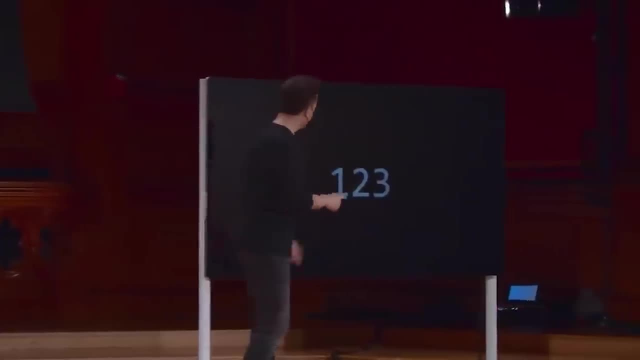 course. In fact, it's one of the best courses I've ever taken in my life. I was absolutely blown away. I came out of this course wanting to consume all the information there is in the world about programming and coding And I was like: I'm going to do this. I'm going 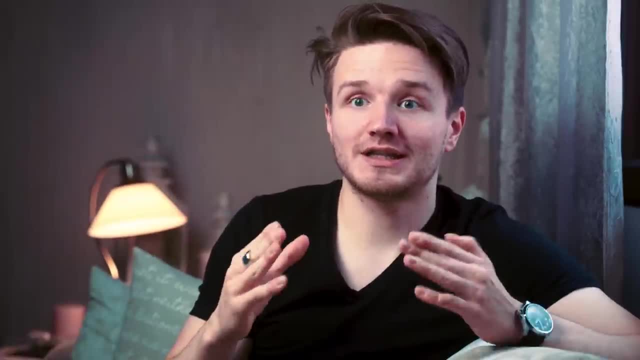 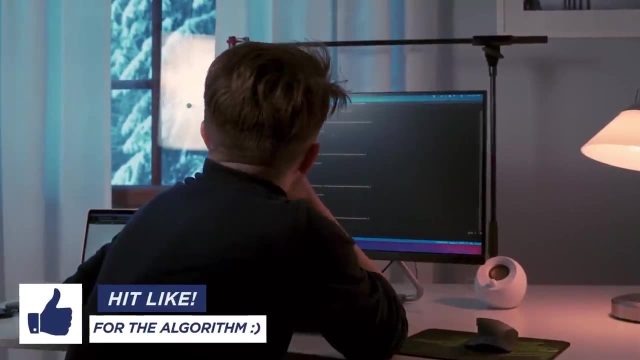 to do programming in computer science. That is how excited about this field I was, And that's when I knew that this was the field I really wanted to go into. CS50 was very challenging. It's hard. Programming is very difficult. The thing is, I really like working. 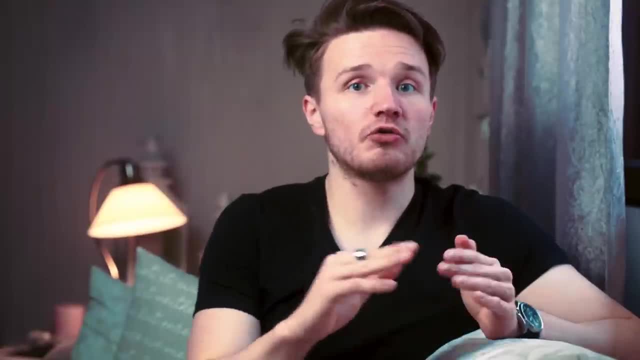 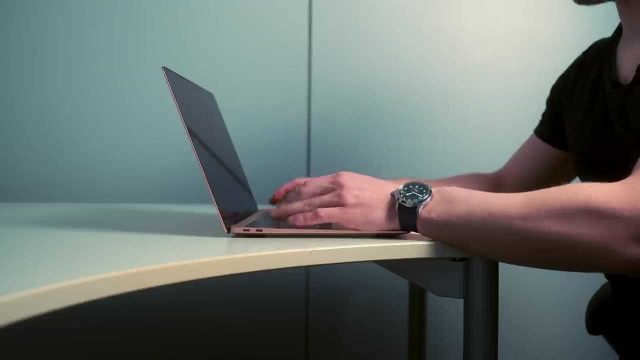 on difficult problems like this And, by the way, this kind of problem solving is not for everyone, And that's completely fine. The problem sets of the course absolutely kicked my ass, but I really embraced the challenge. From this course I learned the C programming. 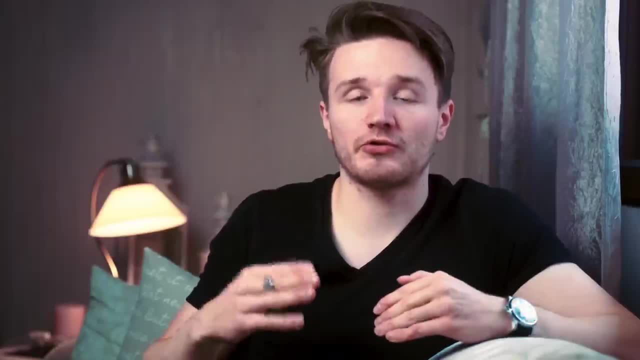 language, which got me introduced to the lower-level implementations of a lot of the functions that you will take for granted in a language like Python, And the course does use Python as well. So I learned a lot about programming and computer science. I learned a lot about 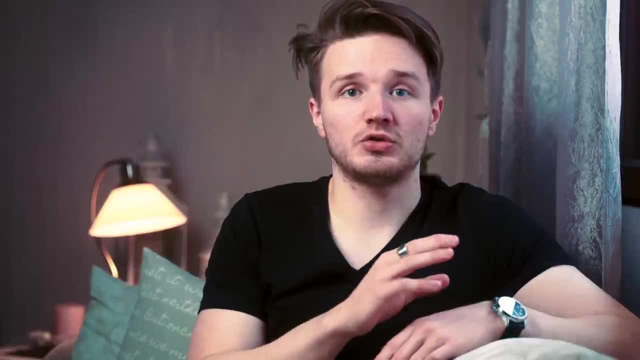 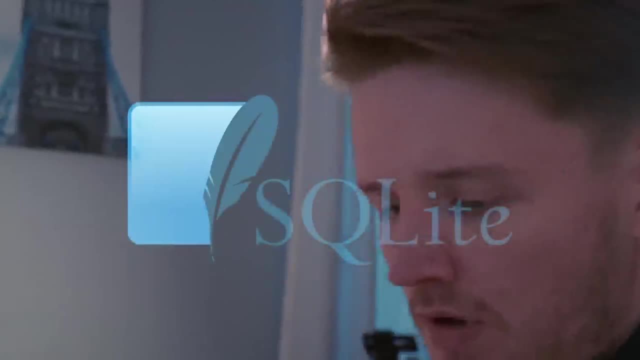 coding as well, So I got even more comfortable with Python. I also got introduced to web programming, which I had already been doing as part of the Odin project. I also got introduced to how to use databases via SQLite. But, most importantly, it taught me the fundamentals. 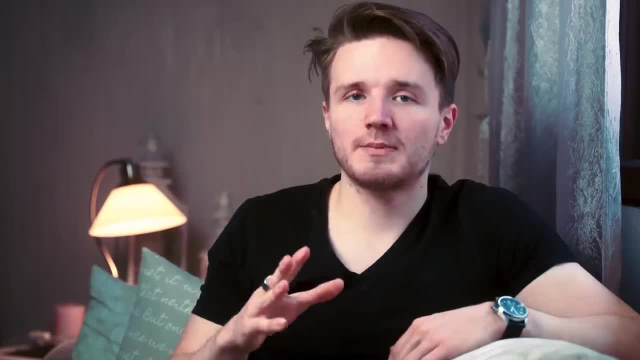 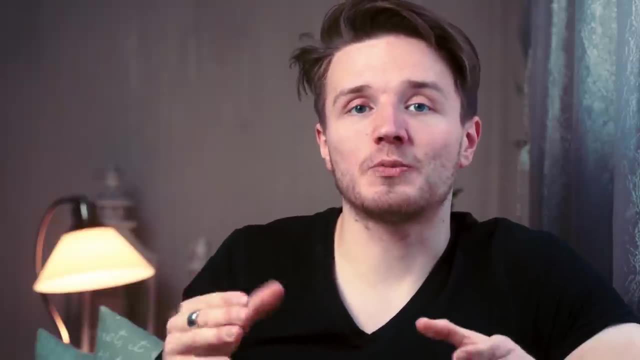 of how computers work at a low level. This is what I feel like: many people learning coding neglect, especially if you're self-taught. But I think it's really valuable to at least get some kind of an understanding of how computers actually work, because that will actually 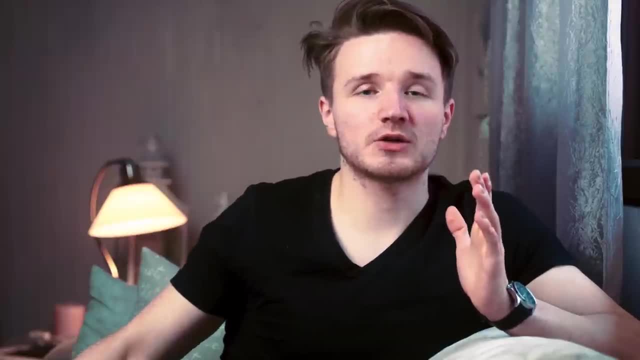 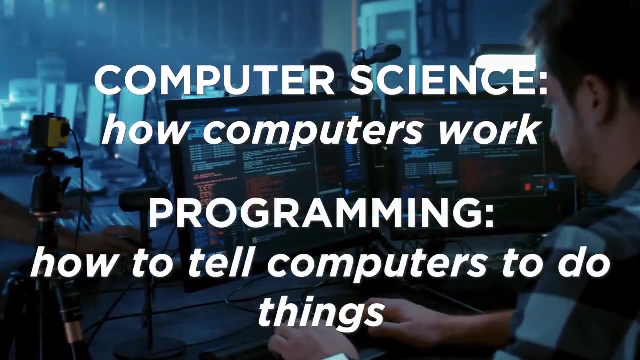 make you a better programmer down the line. And in case you're not aware of the difference, computer science- stuff like that Study- is how computers work, whereas programming is more like how do you practically create program? How do you talk to computers to get them to do stuff? But the better you understand. 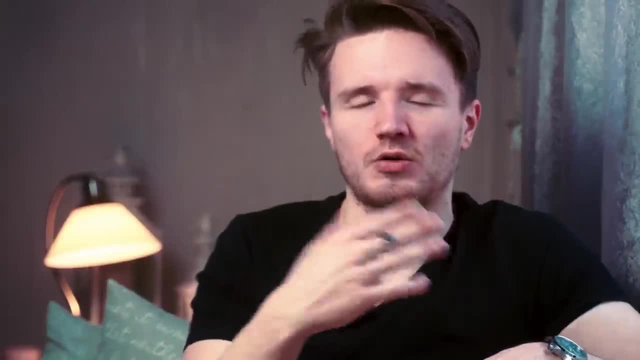 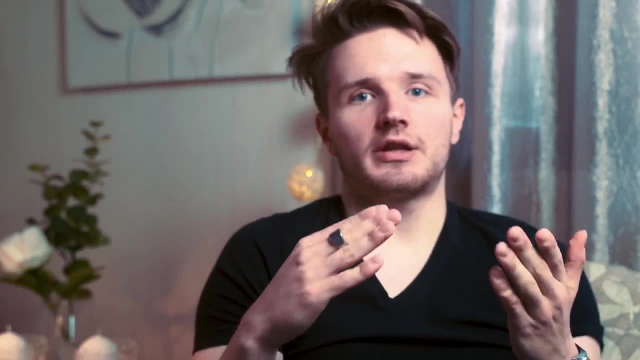 computers, the better you will always be as a software engineer or a programmer. As the final project of CS50, you're going to be building a full-fledged web application using the stuff that you learned in the course. So at this stage you will essentially know. 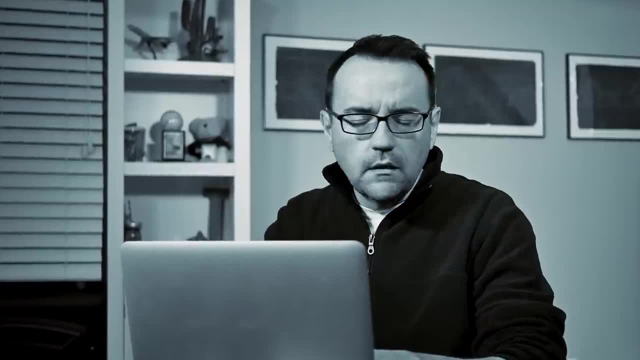 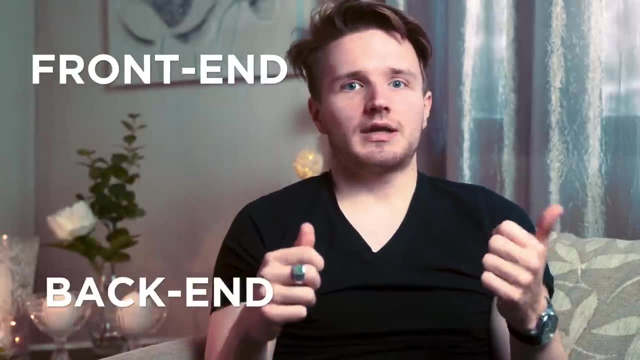 how to code. You'll be able to build very simple things. It'll be a struggle, but you will have an understanding of what it means to build a front-end of a web application And what it means to build a back-end of a website, And what sort of languages are used. 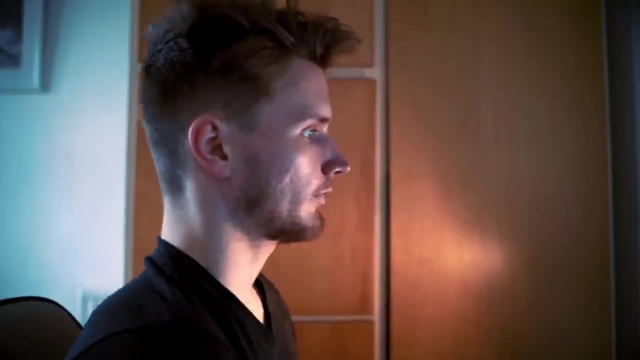 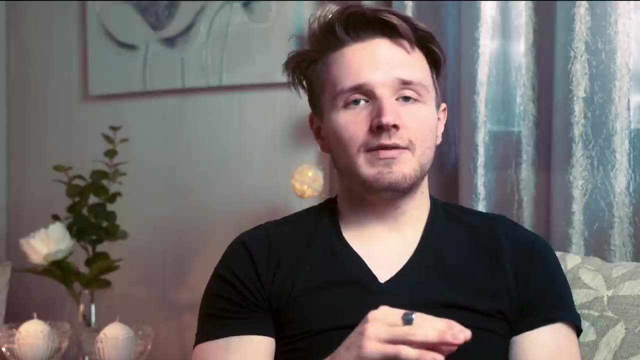 for all of these, And how to actually connect the front-end with a back-end using a framework like Flask, which is the one that you will use in the course. After doing this, before venturing into other areas of programming, I wanted to get even 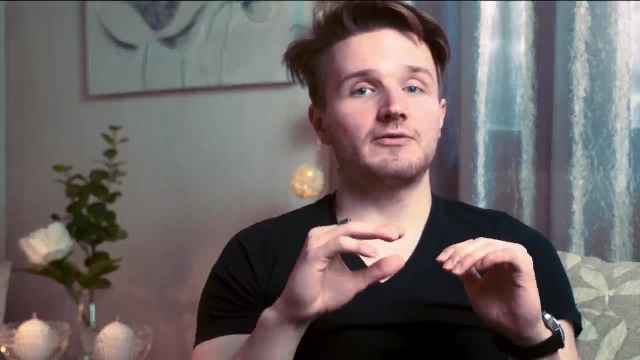 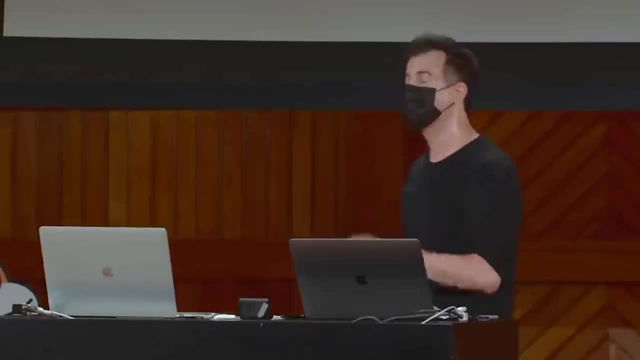 better at web programming specifically, So I did CS50's follow-up course- Web Programming with Python and JavaScript, And this course is essentially a continuation of the extremely engaging and exciting style of CS50, but it's just even more focused on a web programming. 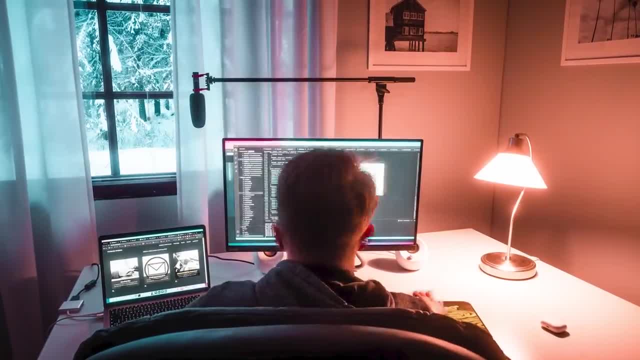 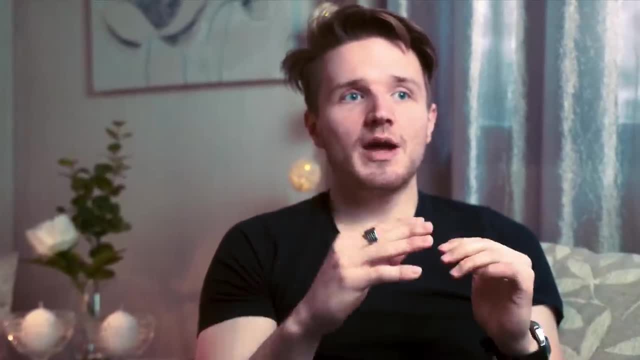 specifically rather than computer science as a whole. And be warned, this one moves at an even faster pace than CS50.. You will know from my CS50 review that CS50 is very hard And the continuation course, CS50 Web, is even harder, Every single week pretty. 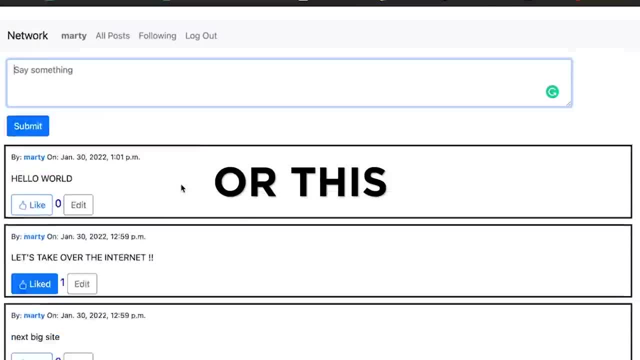 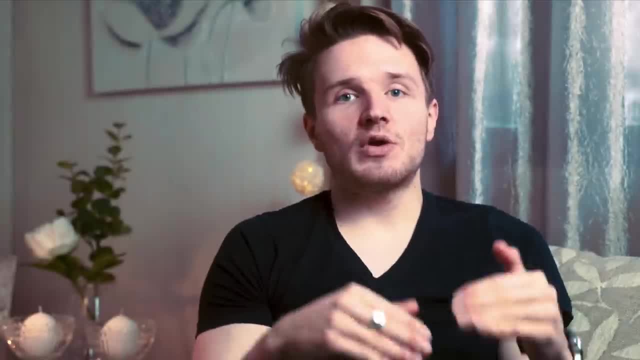 much. you'll be building full-fledged web applications, This time using the Django framework. It will really really push you to get better. But the great thing is that every single week you're building an actual application which you can then put on your portfolio later to. 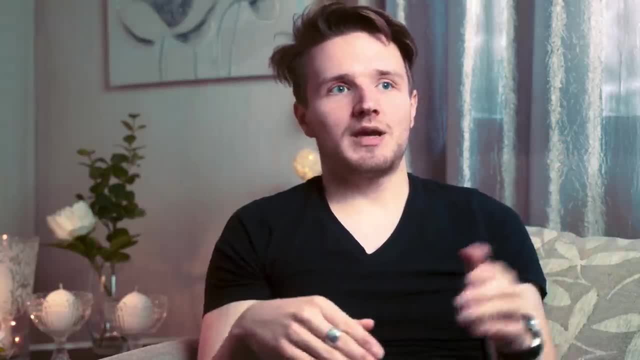 apply for jobs. Again, they are simple compared to the things that you're going to be doing in the future, So I'm going to show you how to build a full-fledged web application using the Django framework. So a lot of the stuff that you'll be able to build if you've worked as a software engineer. 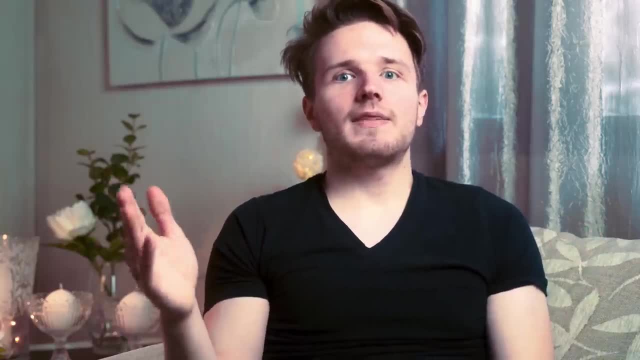 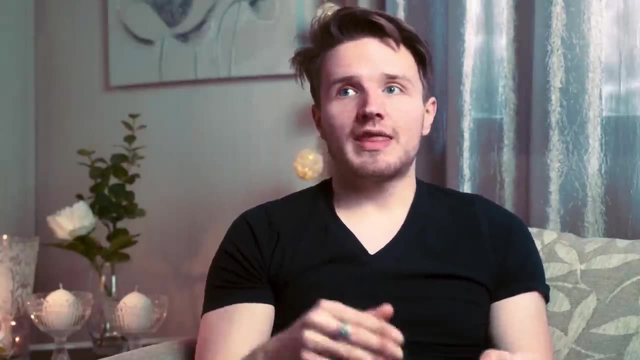 for a long time. but again, for entry-level jobs they don't really require that elaborate stuff. It took me a while, but I came out of this course having a pretty decent understanding of web programming, to the point that now, if I have an idea of building whatever, I 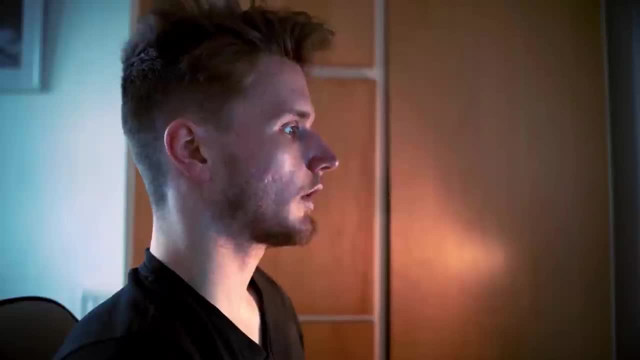 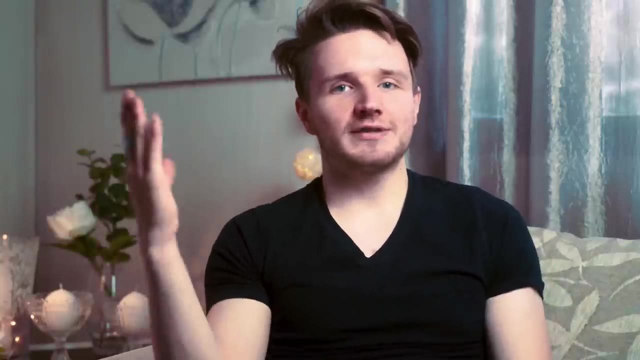 can just go out and figure out how to build it on my own. I don't need a course to hold my hands anymore, And that's really the goal of these courses is to hold your hands to the point where you know just enough so that you can go into the world yourself and build. 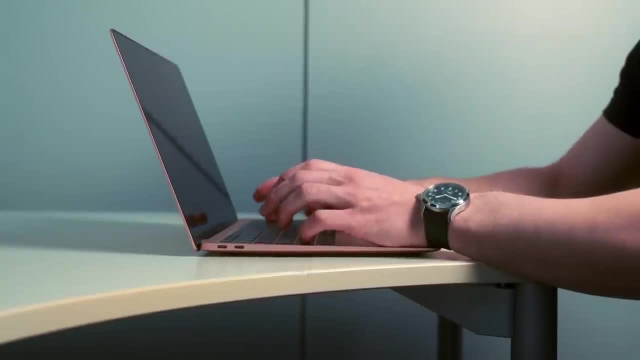 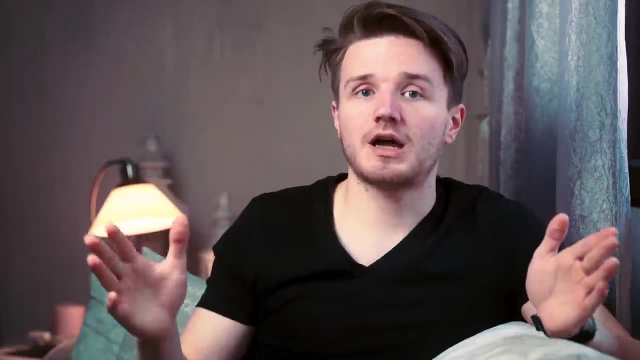 whatever you want to build. So if you do all of these steps, and you do them properly, you will now know how to code. I did this all in around four months. It might take you longer. If it does, that's completely fine. I had a lot of time to put into this. I've been able to work on all of this for 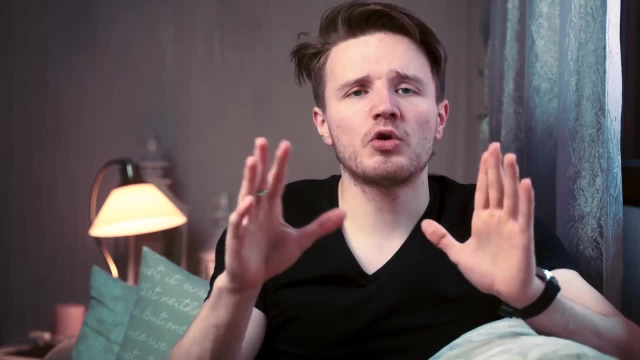 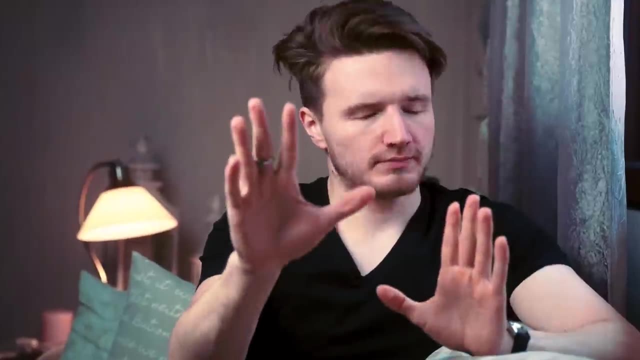 around a couple of hours each day. It's absolutely fine to take your time, But before I get all the experienced software engineer typing on my comments, you know how to create a simple web program. That's nothing. Look, hold on. I understand that coding is. 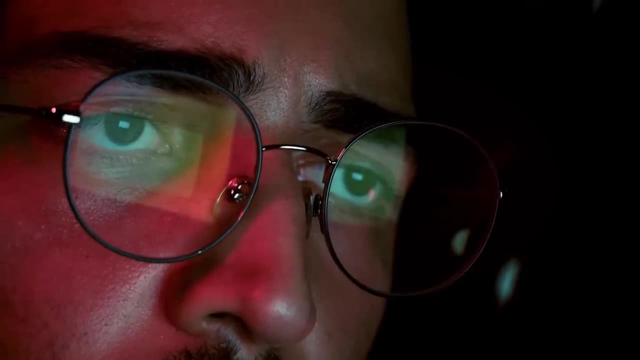 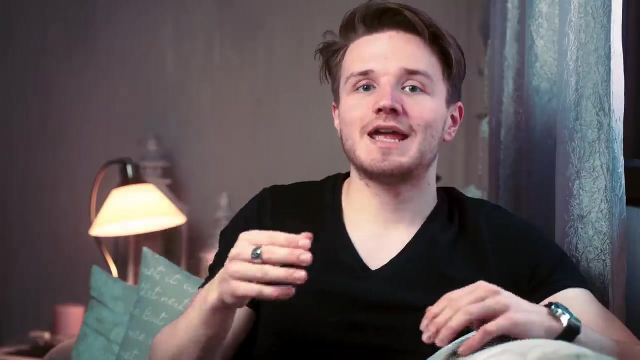 a skill that you will never really master. It's a field where you always need to keep learning new things, because there are always new technologies coming out, software engineering practices change and that kind of stuff. So when I say you will know how to code, I don't. 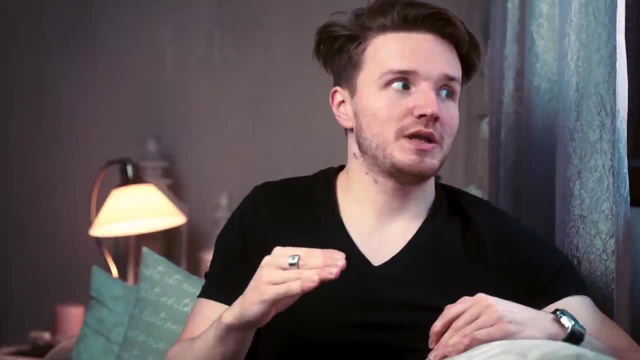 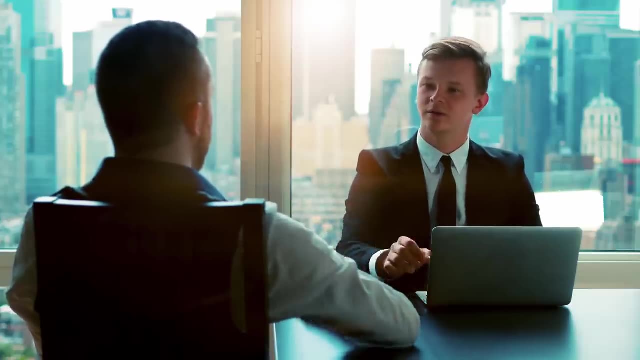 mean that you will be a master. I don't mean that you will be a great software engineer. What I mean is that you will know enough to start creating simple things, and you will know enough to get your foot in the door in the industry than to get your first job In. 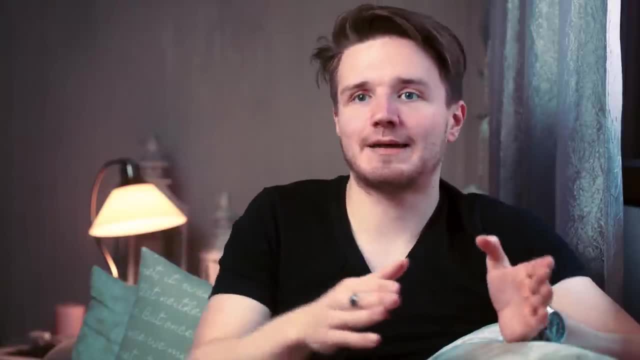 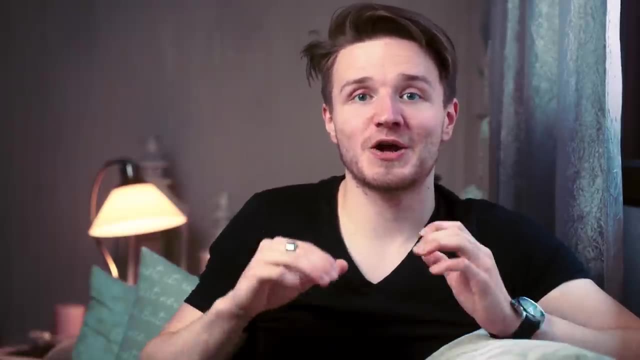 terms of web programming, for example. you will understand what the front end and back end means and how to connect them using a framework like Django or Flask, And you will navigate yourself in the tech world. And that is what I would call the first step of 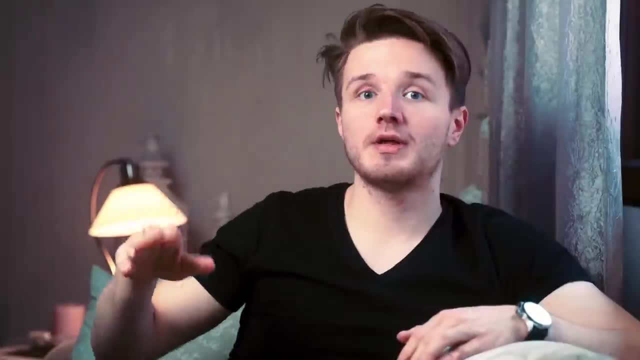 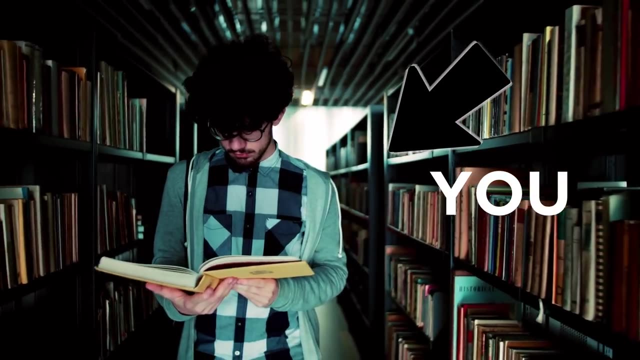 getting into the software engineering industry And then, when you get your first job, that's when you will keep improving down the line. obviously, This field is something where you will need to become a lifelong learner. You need to be someone who likes learning new skills and updating their learning all the time, If that's. 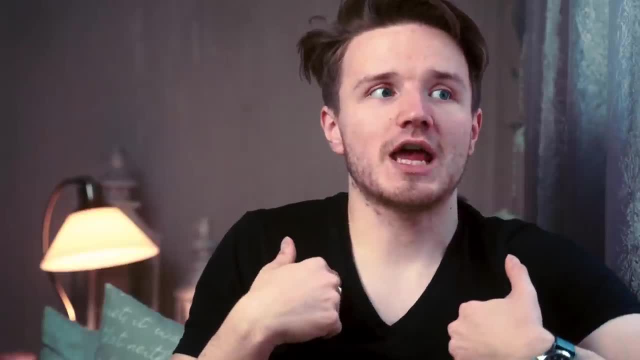 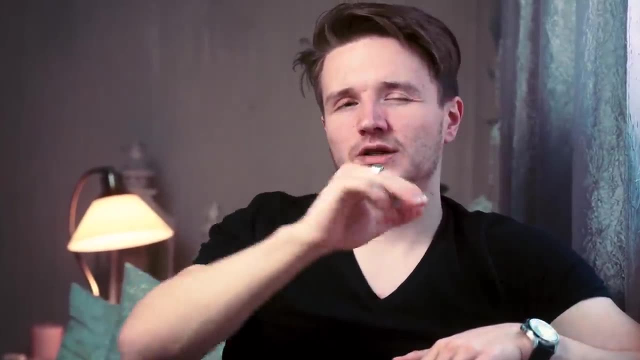 not you, then this field might not be for you. I know it's for me because I love learning new things. That's why I'm so excited about this field. Just keep in mind and think to yourself. You can do something that you want or that you don't want, But I will tell you that in 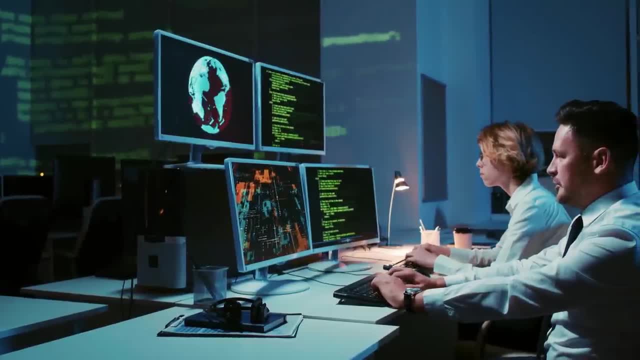 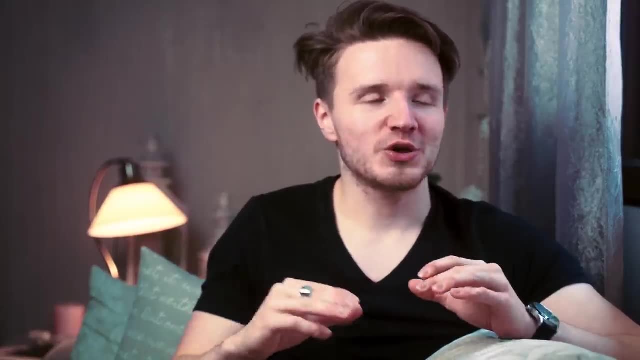 this day and age, coding is sort of the closest thing that we have to a superpower. It's one of the most in-demand skills in the world. So if you just learn enough coding to get your foot in the door, you'll pretty much be good for the rest of your life. There is 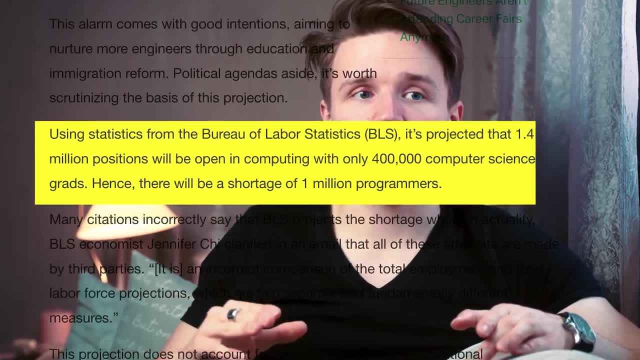 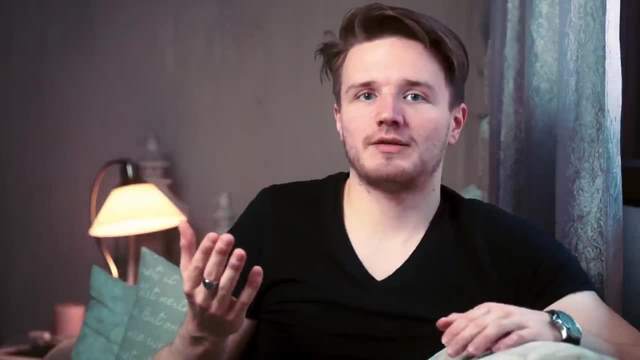 so much demand for these skills. There are so many jobs of software engineers And no, it's not going to be replaced by AI anytime soon. If it does, please kill me. In fact, if you look at any of the predictions from people and my own opinion, they will just. 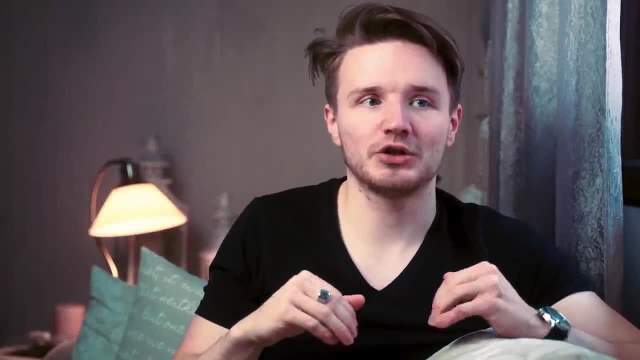 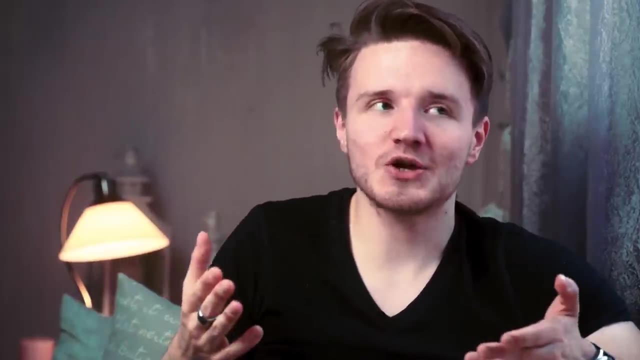 say that there are not enough software engineers in the world to fill up all the positions that are available. So if you learn this skill, you will have something extremely valuable, And it's a pretty good feeling to be able to offer something that's genuinely valuable. 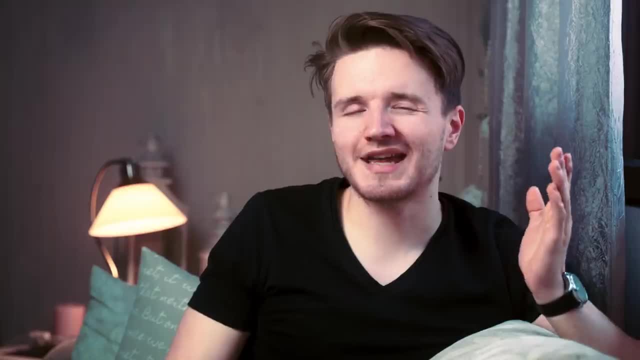 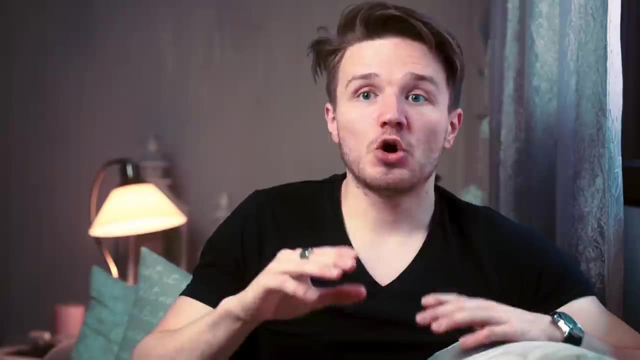 to the world. Okay, so I didn't talk about my software engineering job yet, So here's how that happened. The truth is that I got slightly lucky, because what actually happened is that, during this process that I've described, I did a non-software engineering internship. 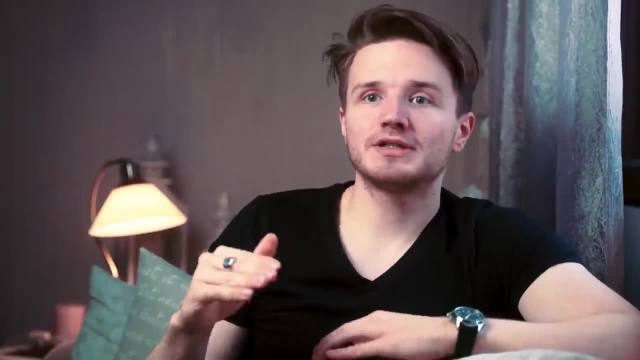 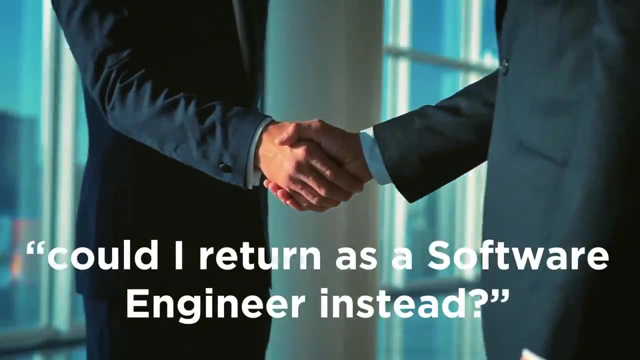 at a big company. It was a business kind of internship And it just so happened that I was in a division that also hired software engineers. I did well in the internship and they wanted to give me a return offer. So I just asked them: Hey, will it be possible? 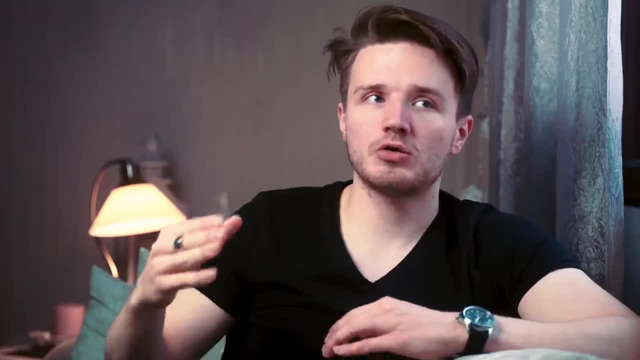 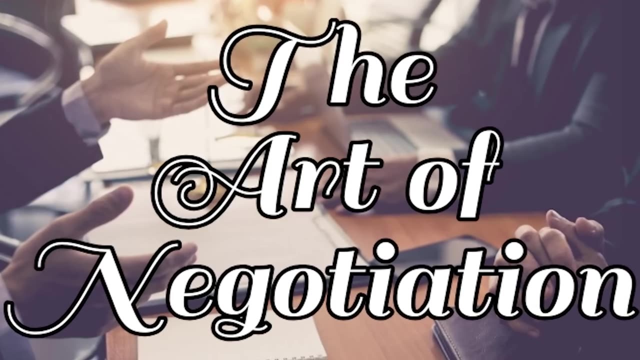 to get that return offer as a software engineer, Because actually I've been learning coding, So I was basically just able to convince them of my potential and motivation as a coder person to get them to give my return offer as a software engineer. So you could say that: 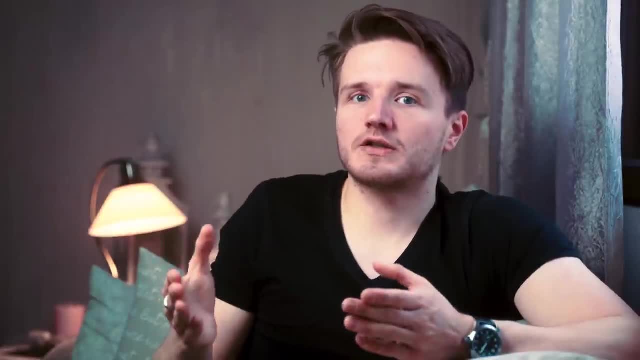 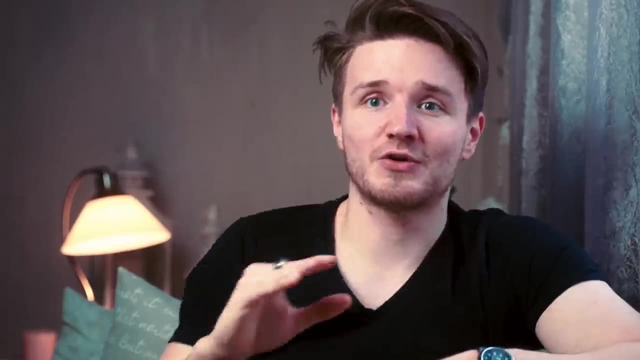 I got slightly lucky, But what this goes to show is that you should always ask, You should always try before you think you're ready. At this point I was around two months into my process. I certainly didn't think I knew enough coding to actually apply for software engineer jobs. 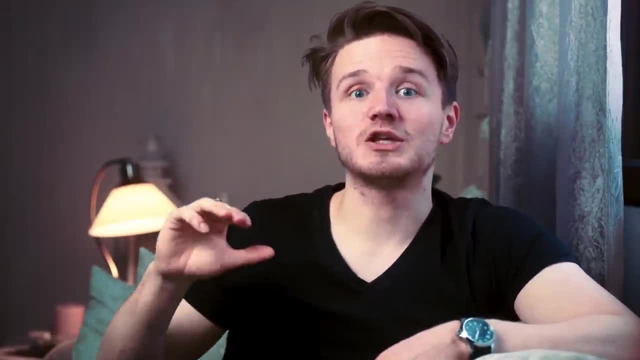 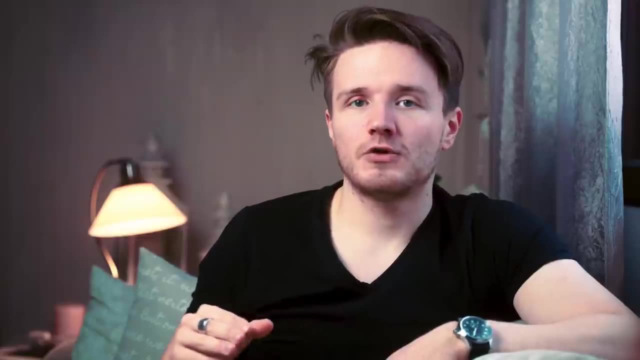 directly. But what this goes to show is that try before you think you're ready. You never know what's going to happen. And even if I hadn't got this job, I think with my skills now I would certainly be able to apply for software engineer jobs directly. I have a.